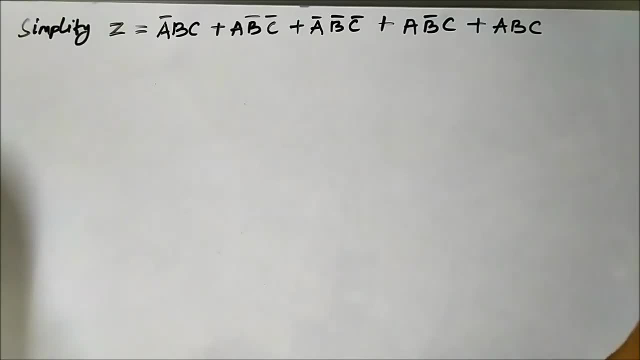 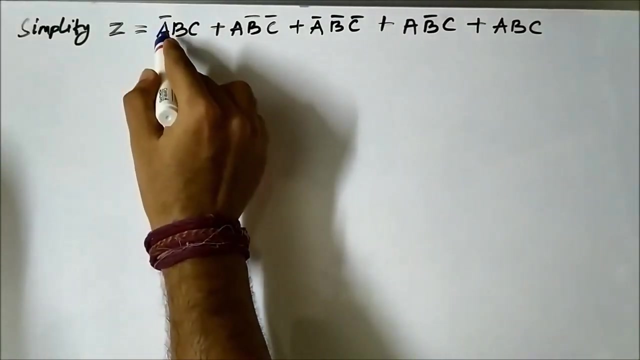 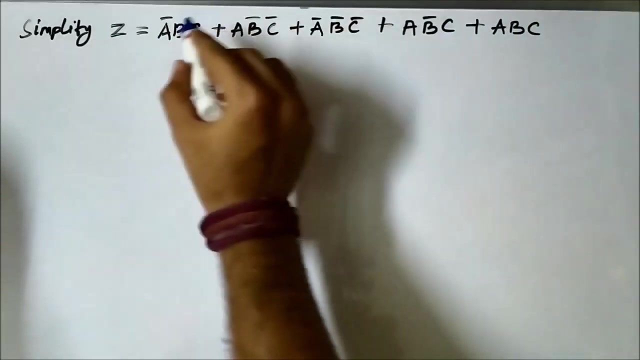 We have to identify common terms. That is our first objective While solving any, simplifying any Boolean expression. first we have to identify the patterns, the common terms. So here, look at this term a, bar, b, c and this abc. Here both the terms have b c in common. Here also it is b c there. and 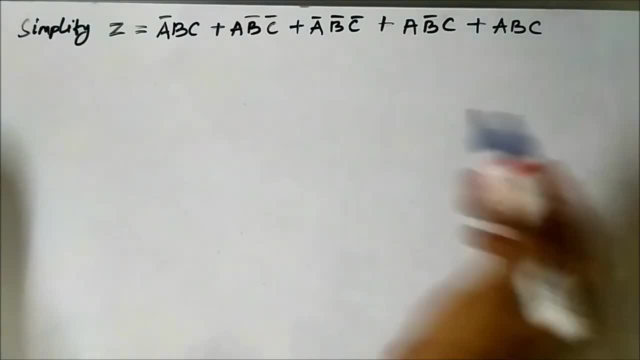 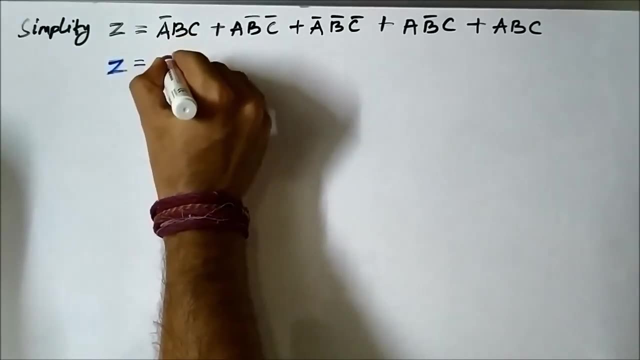 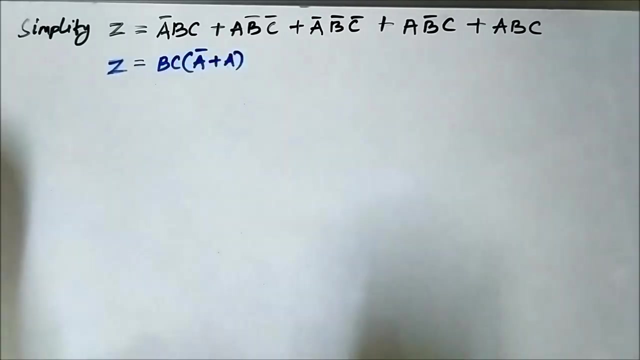 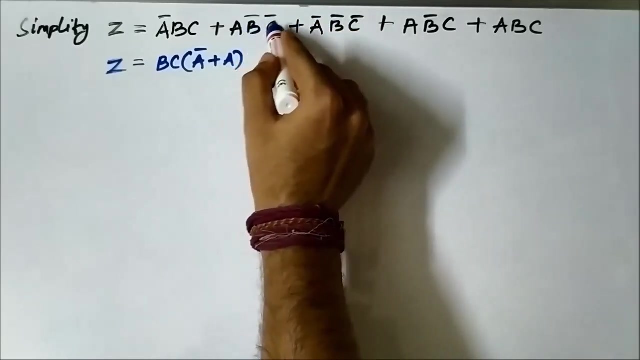 here also there is b c there, So let us take that as common. So it will be b c into a bar plus a. Now let us identify other things here In these two terms, b bar, c bar, b bar, c- bar is common. 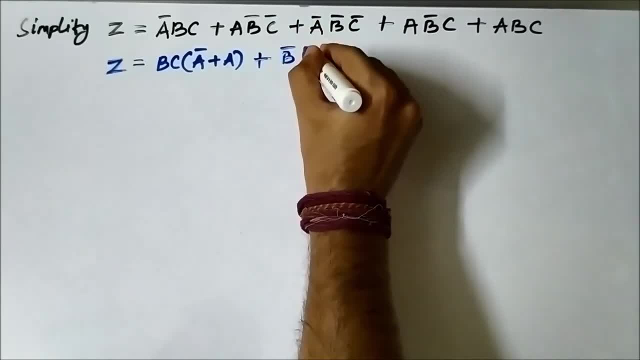 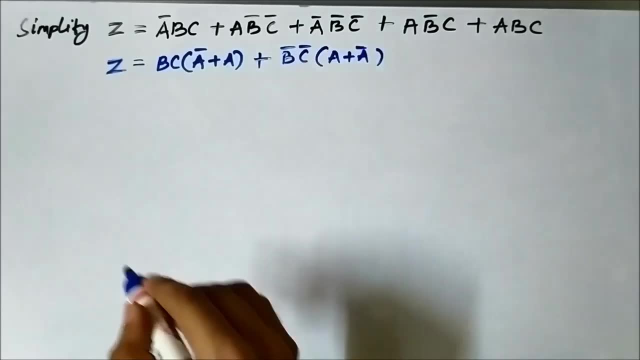 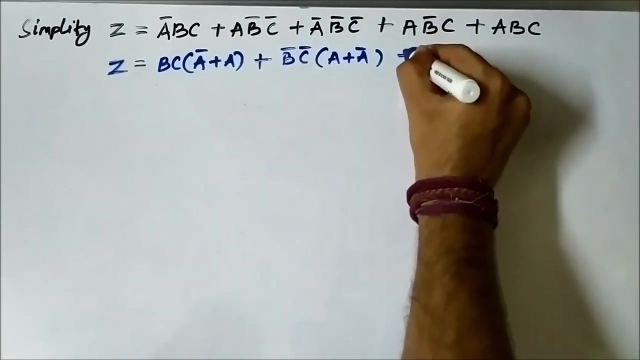 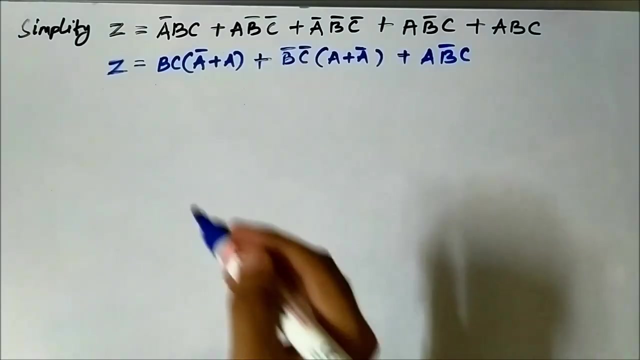 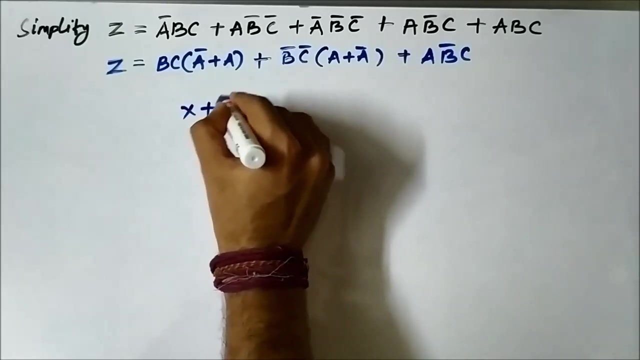 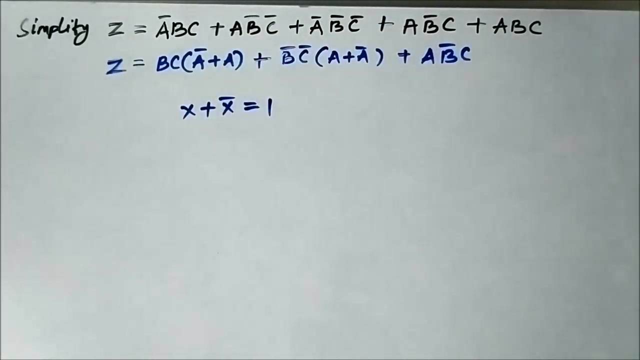 So we can write b bar, c bar into a plus a bar. Now these two, and these two are gone. remaining is this: a b bar. Now, as per the OR rule, we know that any boolean variable, OR with its complemented variable- means its complemented version- will give us 1.. 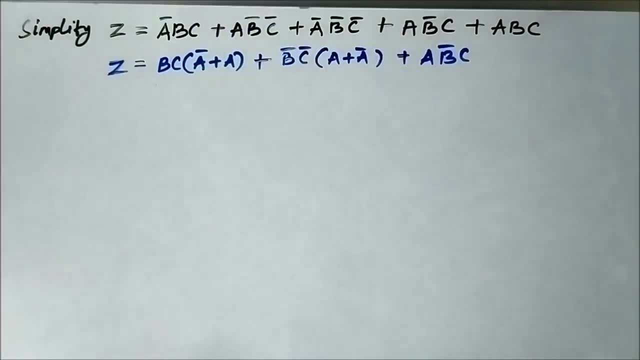 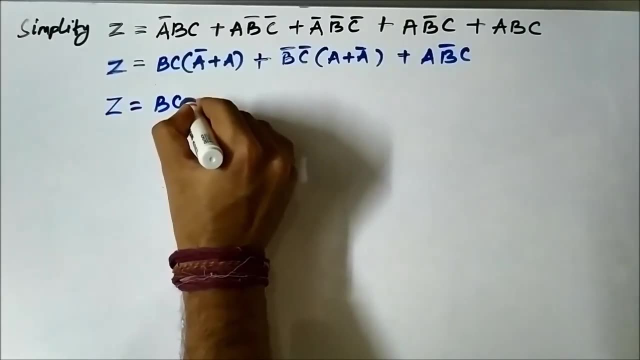 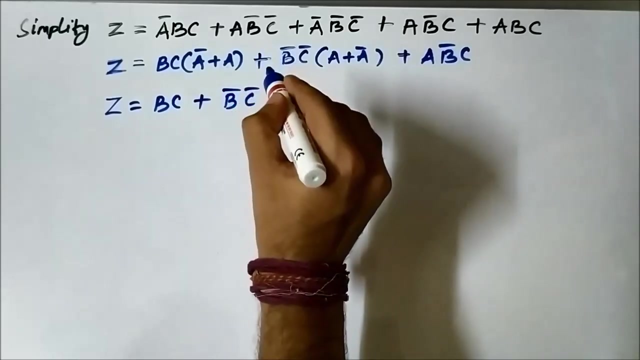 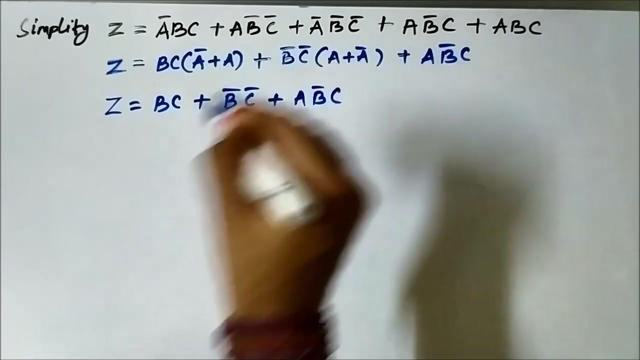 So we will apply that here. So a plus a bar, a plus a bar will give us 1.. So it will be z is equal to bc into 1, or we will simply leave it as bc plus b bar c, bar plus a b bar c. 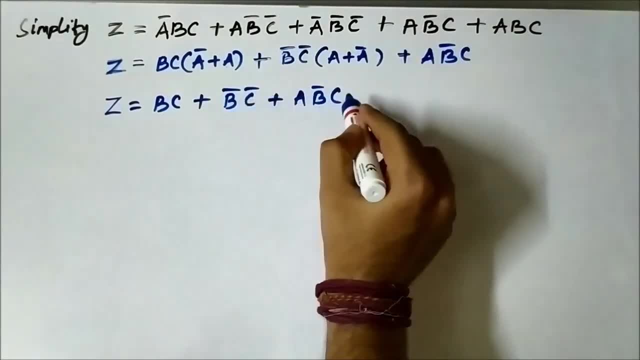 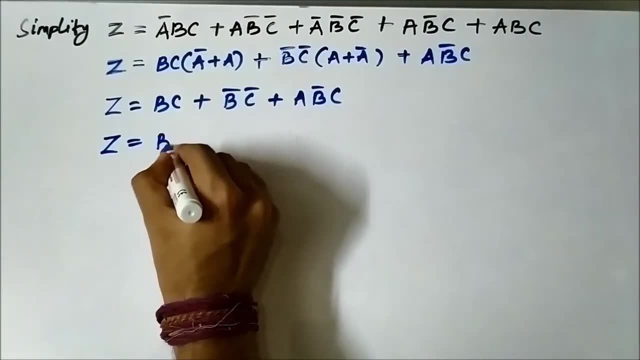 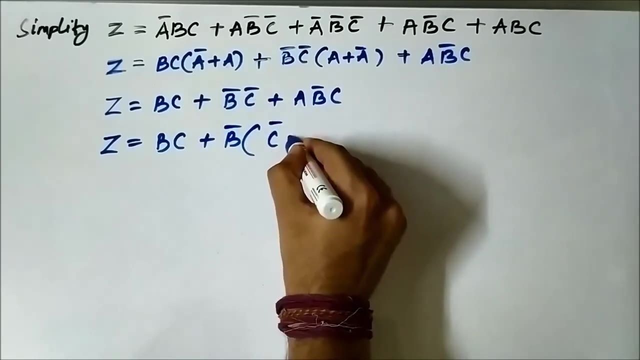 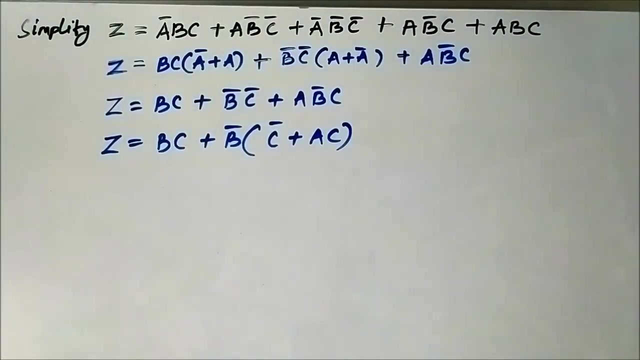 Again, here in these two terms b bar is common, So let us take b bar as common. So it will be bc plus b bar, c bar plus ac. Here we can apply another rule, the absorption rule we can apply, which says that x plus x. 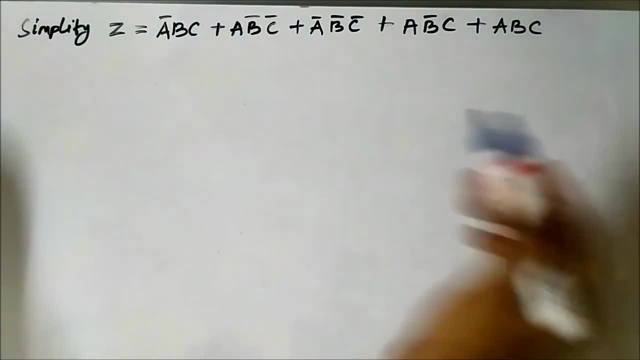 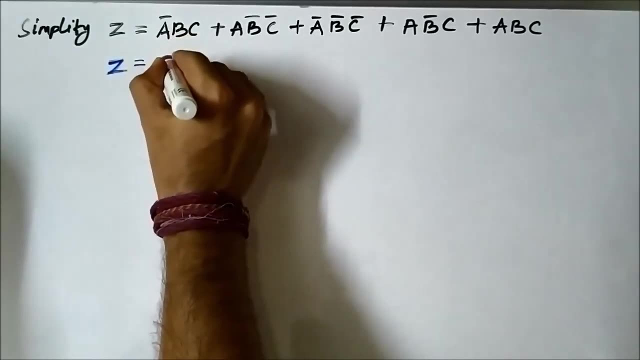 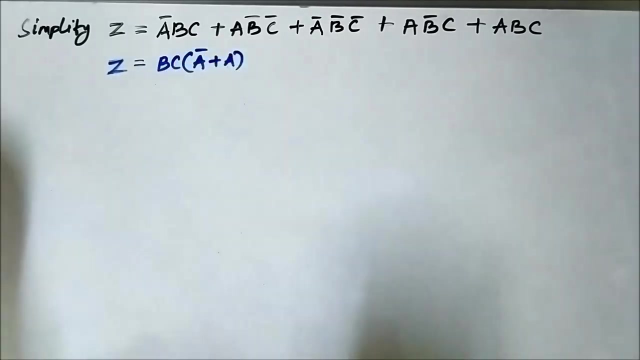 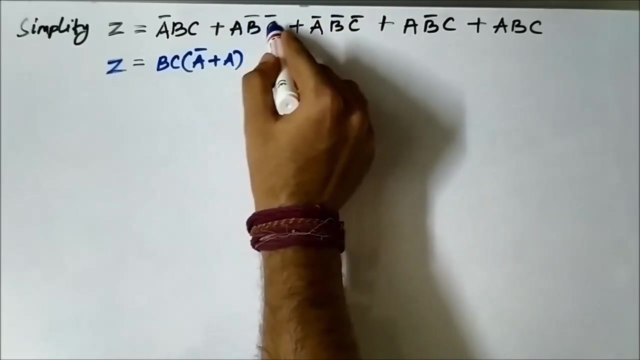 here also there is b c there, So let us take that as common. So it will be b c into a bar plus a. Now let us identify other things here In these two terms, b bar, c bar, b bar, c- bar is common. 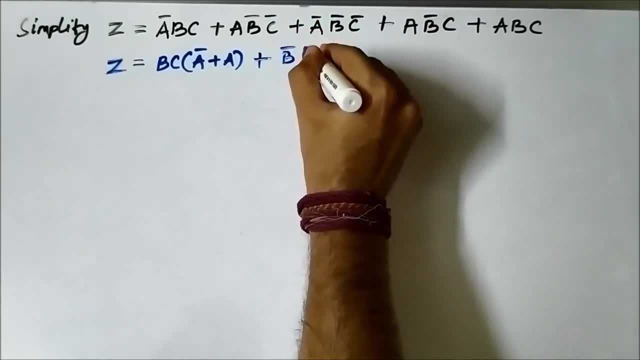 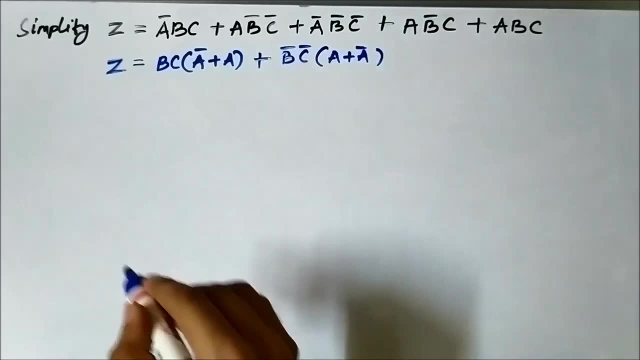 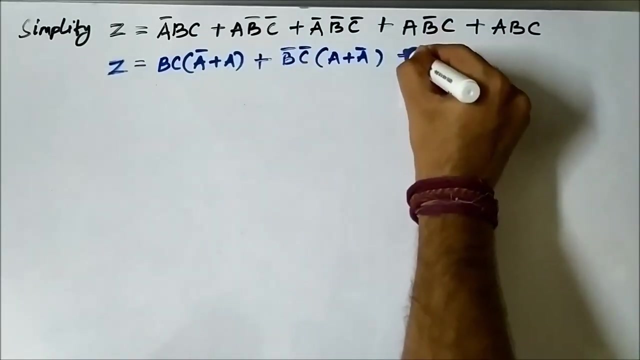 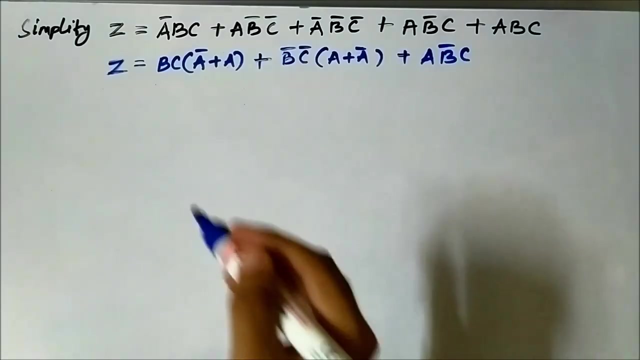 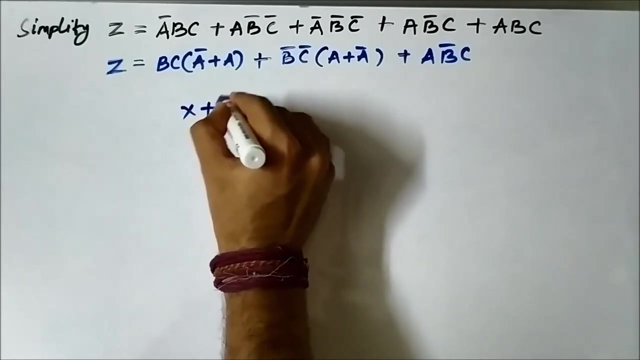 So we can write b bar c bar into a plus a bar. Now these two, and these two are gone. Remaining is this: a b bar c. Now, as per the or rule, we know that any Boolean variable or with its complemented, 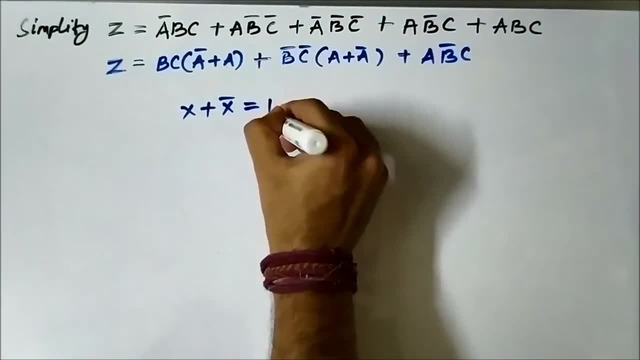 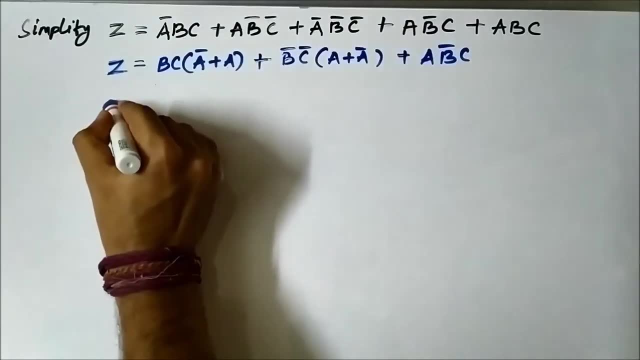 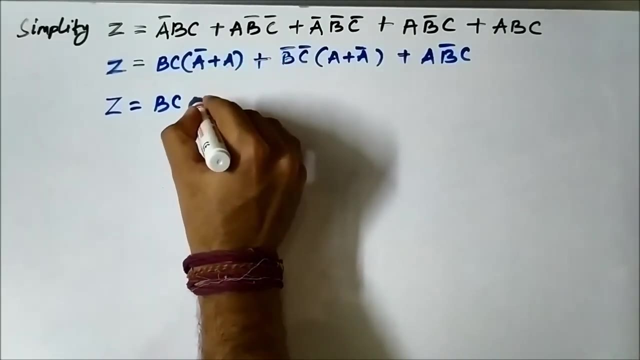 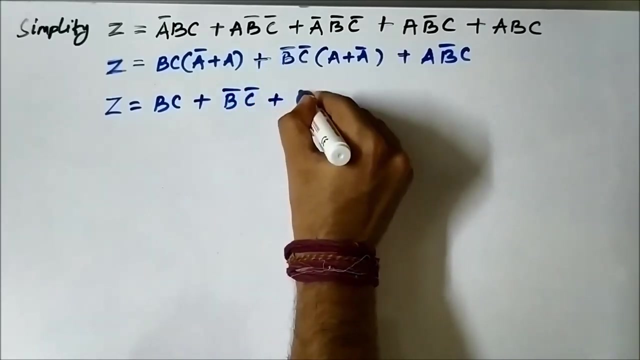 variable means its complemented version will give us 1.. So we will apply that here. So a plus a bar, a plus a bar will give us 1.. So it will be: z is equal to b, c into 1, or we will simply leave it as b, c plus b bar, c, bar plus a, b bar c. 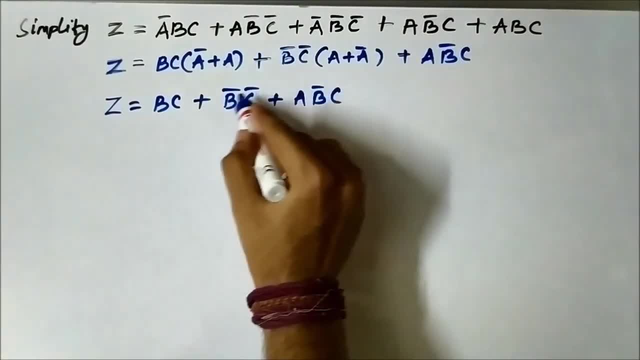 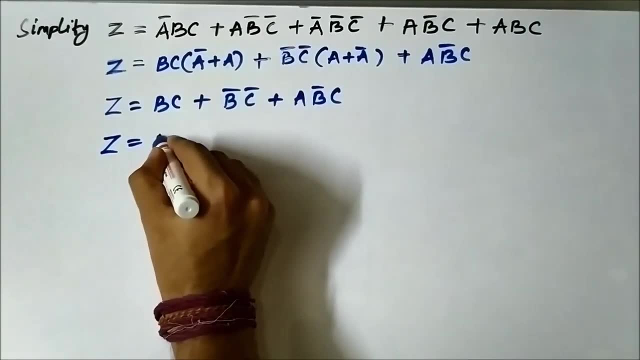 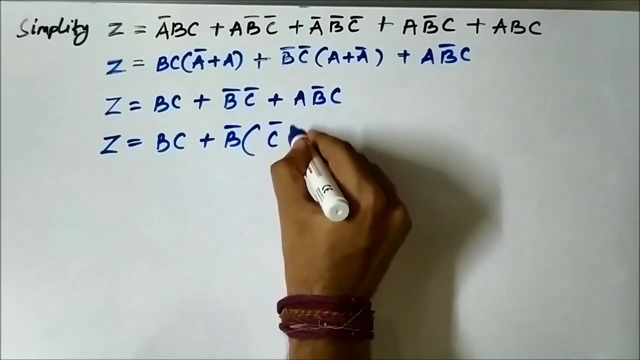 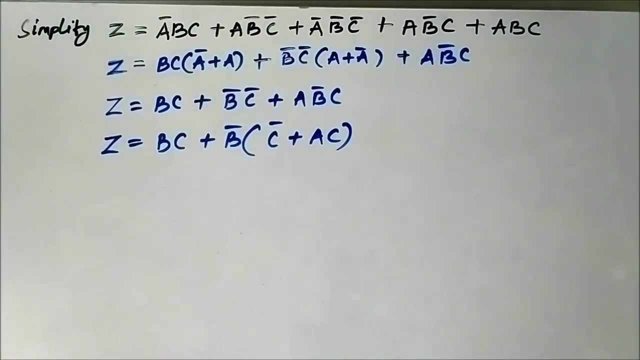 Again here, in these two terms: b bar is common, b bar is common. So let us take b bar as common. It will be b c plus b bar, c bar plus a c. Here we can apply the another rule, the absorption rule, we can apply. 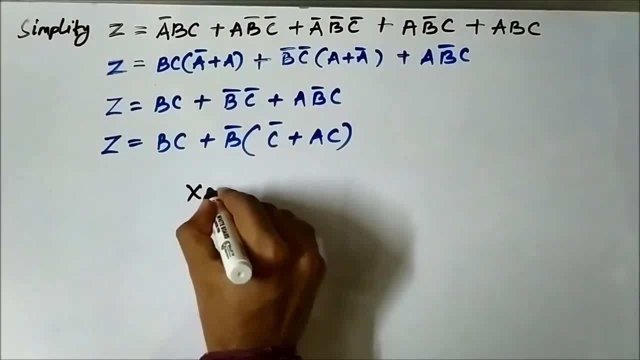 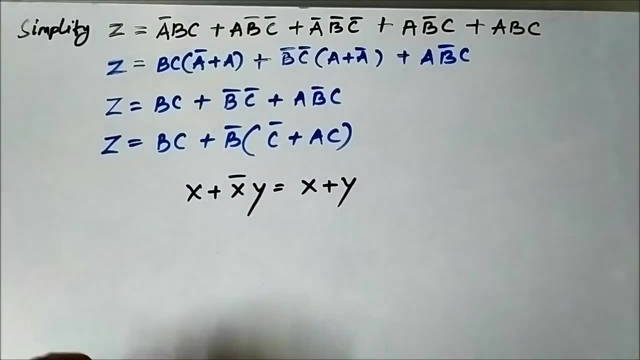 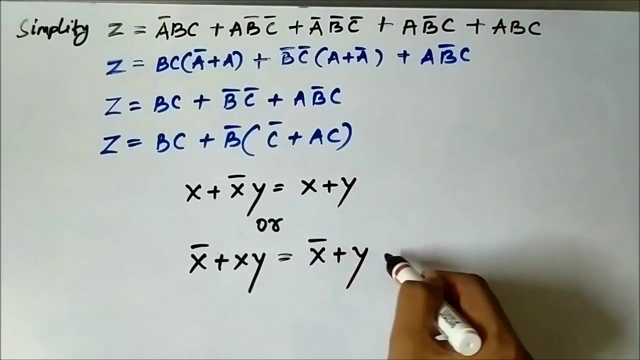 which says that x plus x bar y is equal to x plus y. or we can write it as: x bar plus x y is equal to x bar plus y. So this rule can be applied here: x bar plus x y equal to x bar plus y. So here: c bar plus c, a, a, c or c, a same thing. 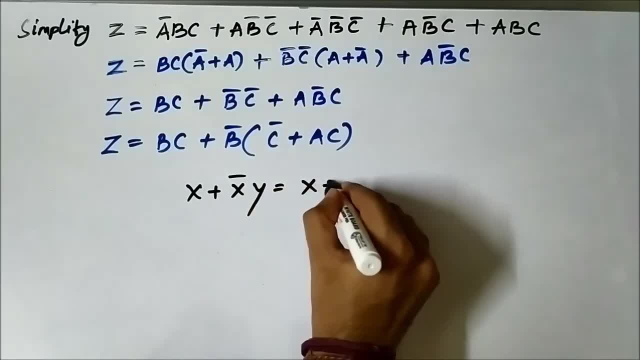 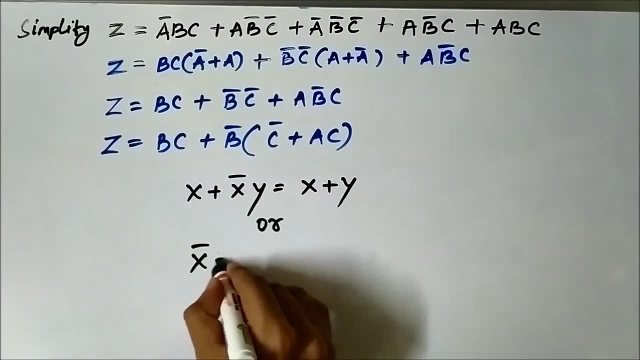 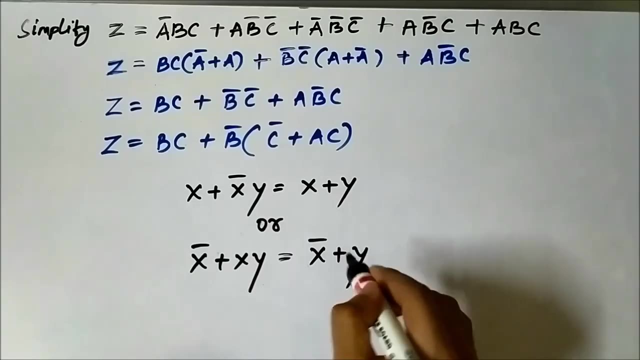 bar y is equal to b, So x plus y. or we can write it as: x bar plus x y is equal to x bar plus y. So this rule can be applied here: X bar plus x y equal to x plus y. So here c bar plus c a. 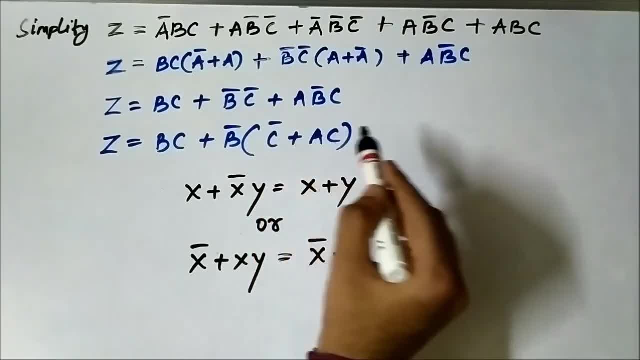 ac or c a, it is same thing. C bar plus c a will simply be c bar plus c a. So c bar plus c a is equal to a bar plus c y. Let us take that here and write it down. Give it a name which is x bar plus x y. 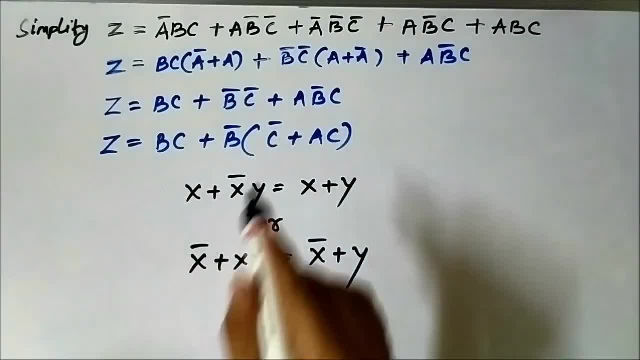 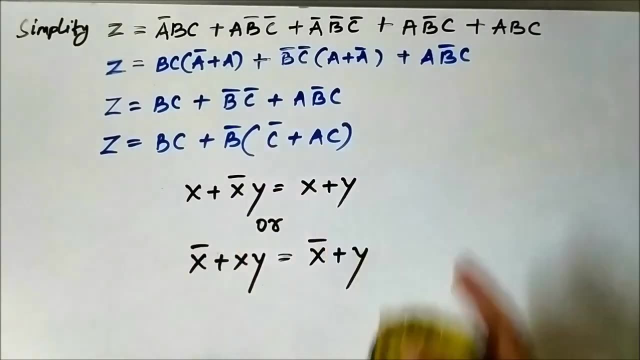 So x bar plus x y equal to a bar plus y plus a. So this will become c bar plus a using this rule, I have already posted the video related to the Boolean algebra rules, So please check out that video. So we will apply this rule here. 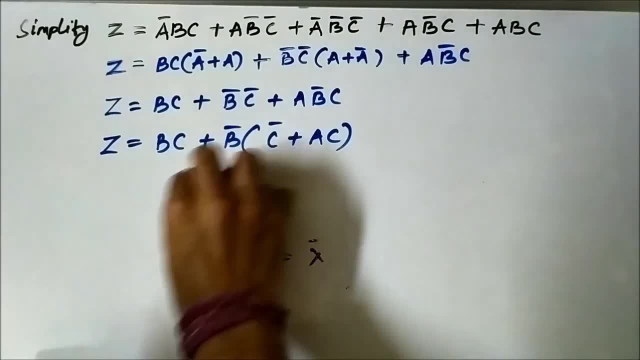 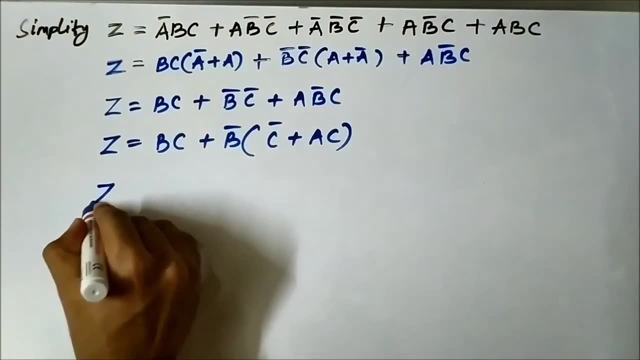 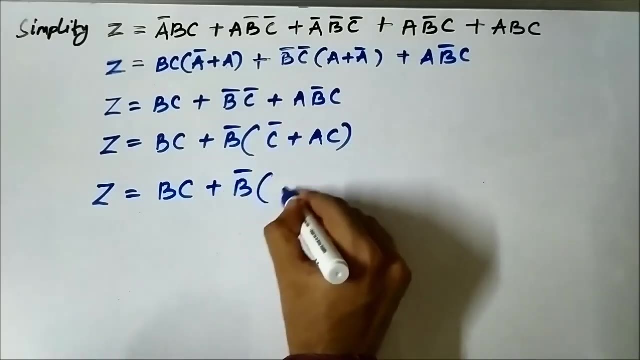 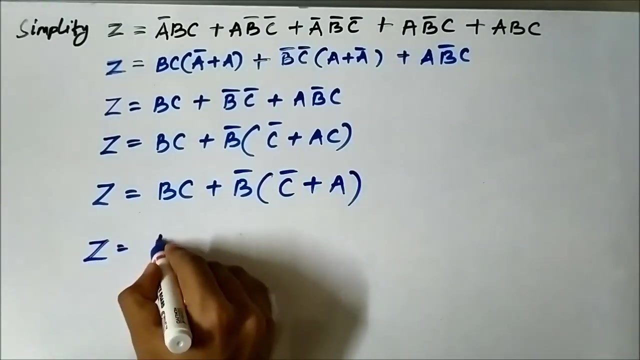 So it will become c bar plus a. So here it will be. z is equal to b, c plus b bar into c bar plus a, So it will become the final expression. I do not think we can simplify any further, because there are no more. 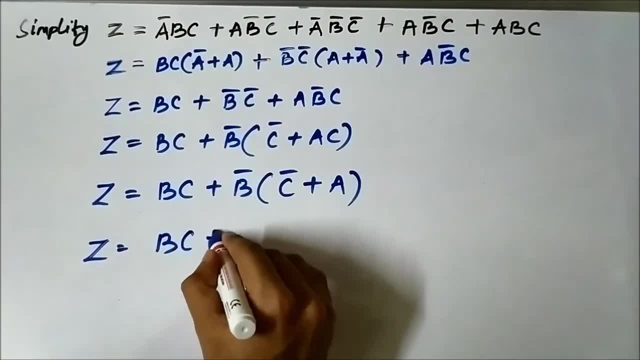 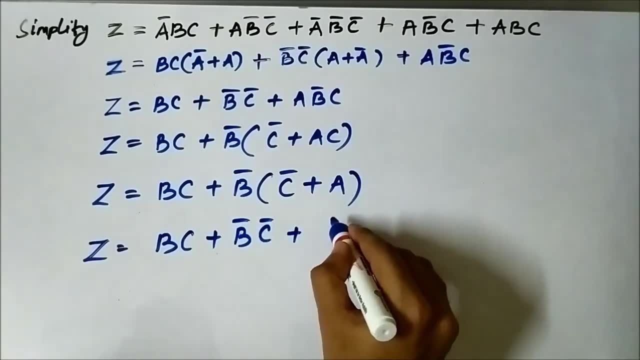 Common terms. Let us see b c plus b bar, c bar plus b bar or a b bar. Should write it in alphabetical order. Now let us see if there is any common term coming which we can apply in Boolean algebra. No, no, This is the final expression Now. 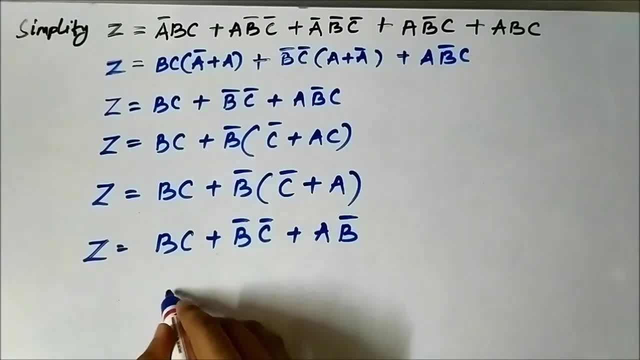 do Do not make this mistake here, that b c plus b bar, c bar is equal to 1.. Do not make this mistake, because here the individual variables are complemented, The whole expression is not complemented. If it would have been like this: b c plus b c, whole bar, then it would have been 1.. 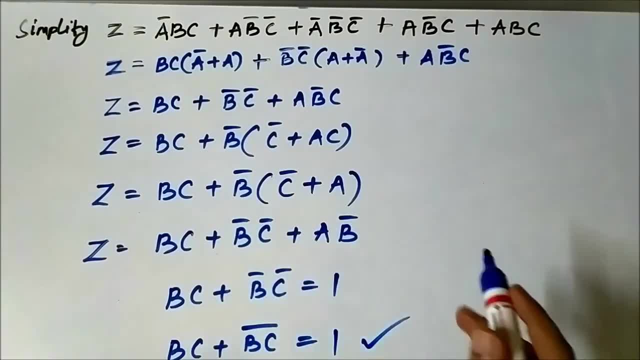 Okay, But here, in this case, the individual variables are complemented, So this is wrong. Sometimes, in a hurry, students make this mistake. Okay, It is natural for beginners. So you avoid this. You just be a little bit careful about that, Okay So 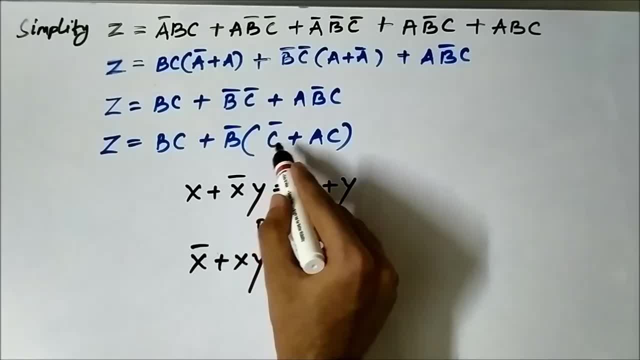 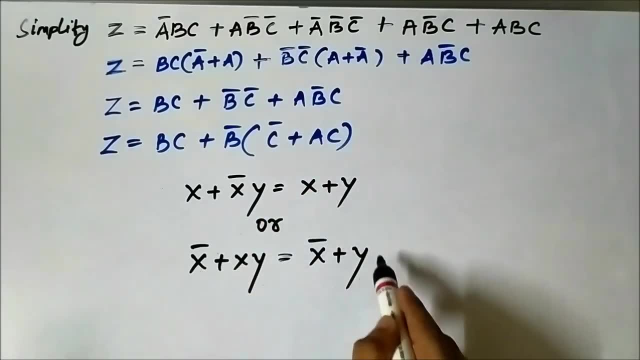 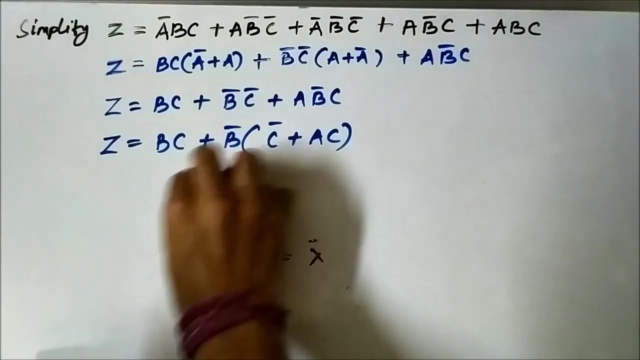 c bar plus c a will simply be c bar plus a. So this will become c bar plus a. using this rule, I have already posted the video related to the Boolean algebra rules. Please check out that video. So we will apply this rule here. So it will become c bar plus a. So 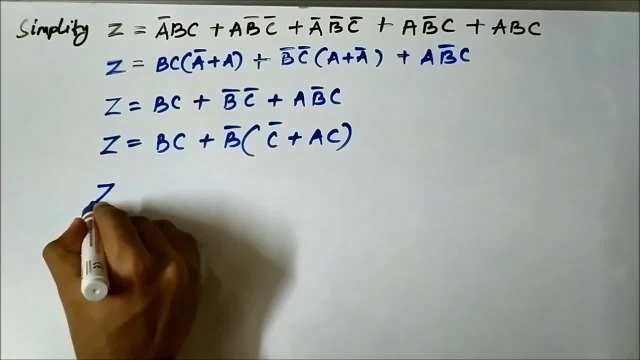 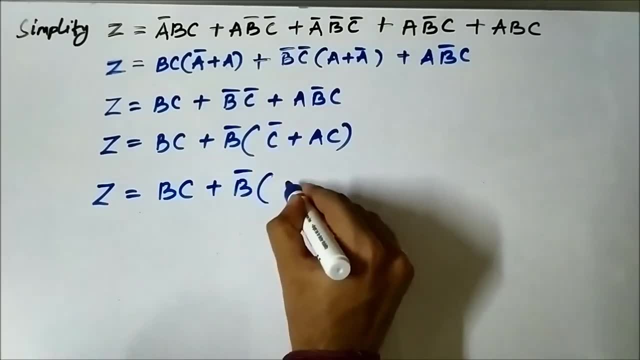 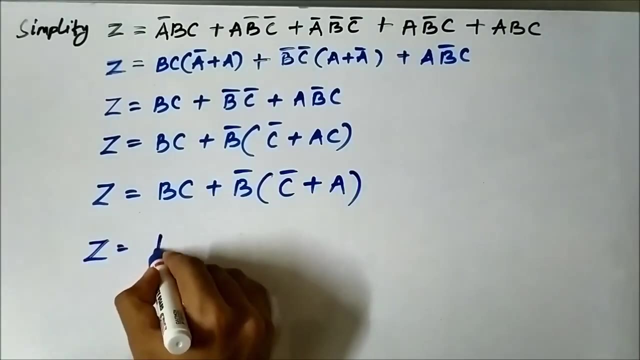 here it will be: z is equal to b c plus b bar into c bar plus a, So it will become the final expression. I do not think we can simplify any further because there are no more common terms. Let us see: b? c plus b bar, c bar. 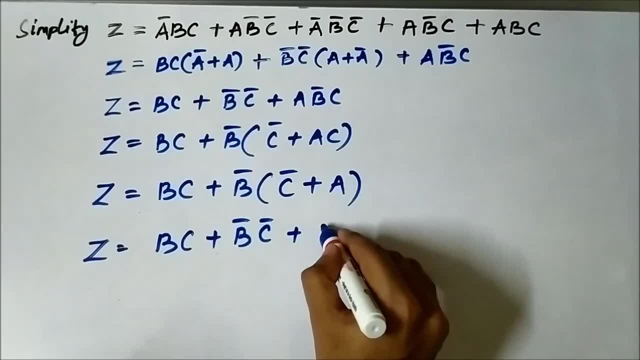 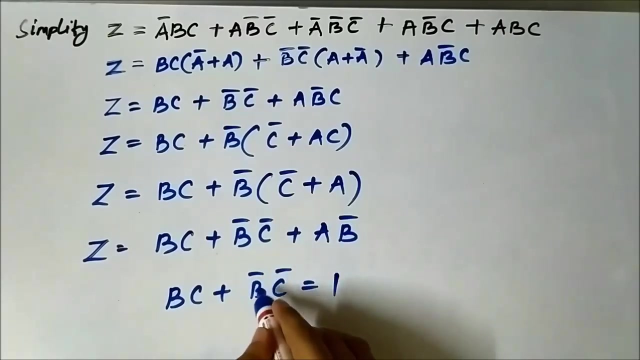 This is the final expression. Now do not make this mistake here- that b? c plus b bar, c bar. So this is the final expression. Now do not make this mistake here- that b? c plus b bar, c bar is equal to 1.. Do not make this mistake, because here the individual variables are complemented. 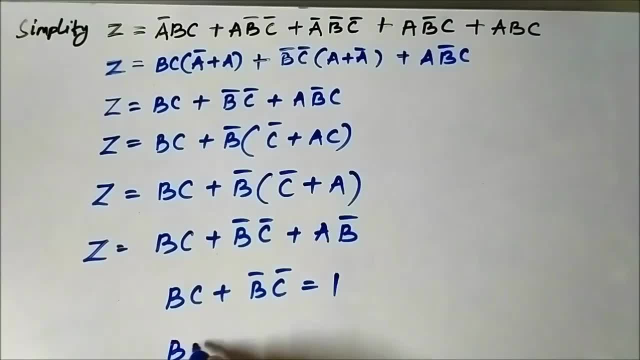 The whole expression is not complemented. If it would have been like this: b c plus b c, whole bar, then it would have been 1. But here, in this case, the individual variables are complemented. So this is wrong. Sometimes, in a hurry, students make this mistake. It is natural for beginners. 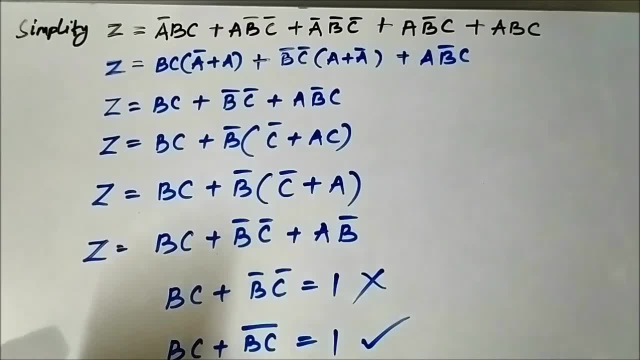 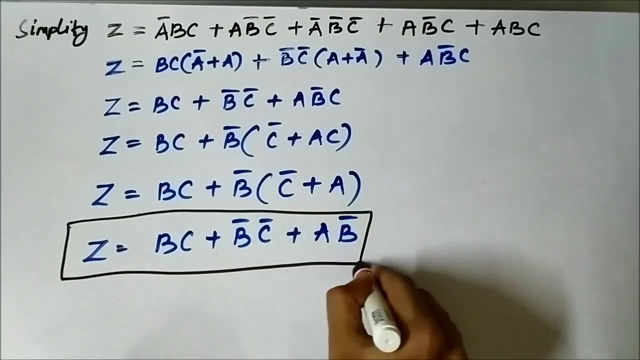 So avoid this. You just be a little bit careful about that. So this is the final Boolean expression. z is equal to b c plus b bar, c bar or a b bar- You can write it in whichever way you want. So, while solving or simplifying any Boolean expression, the first thing that 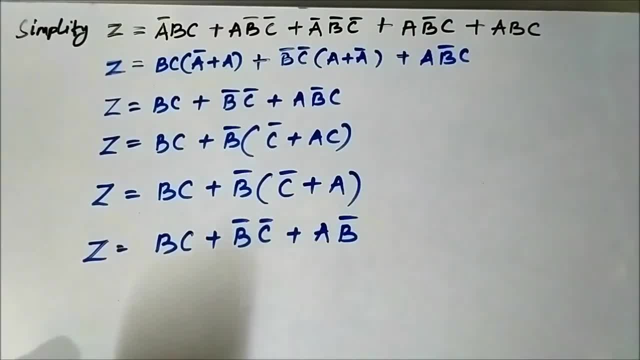 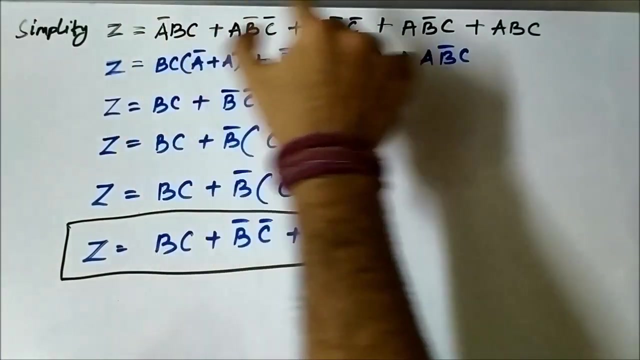 this is the final Boolean expression. Okay, Z is equal to b c plus b bar, c bar or a b bar. Okay, You can write it in whichever way you want, Okay. So, while solving or simplifying any Boolean expression, the first thing that you have to take care is to identify common 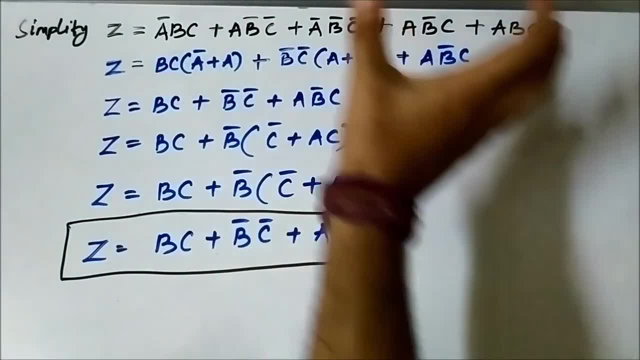 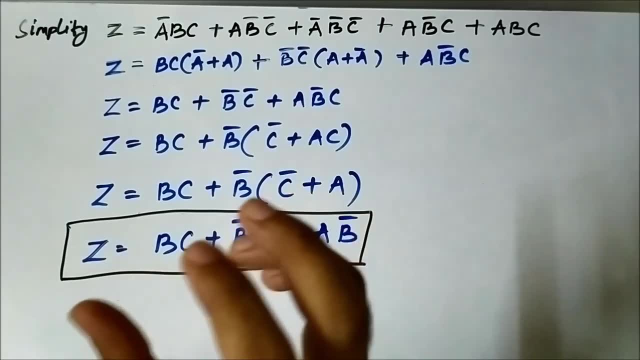 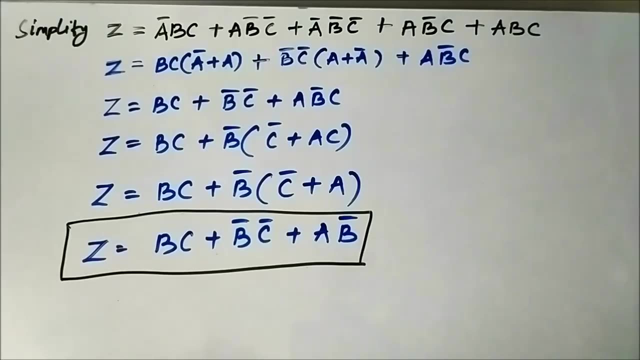 terms in the Boolean expression, Then arrange them in a particular manner where you can apply the Boolean algebra rules. Okay, The simplification rules. So for that, you have to be crystal clear about the rules, You have to remember them. Then keep on simplifying. 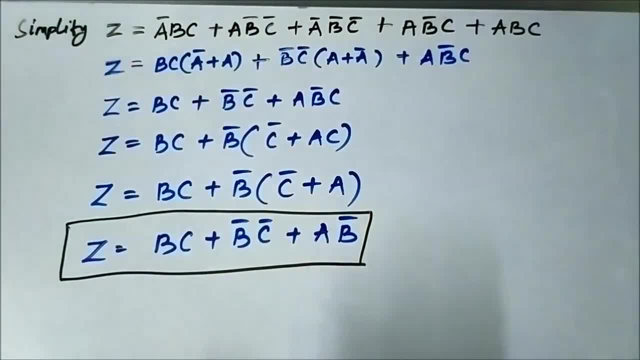 Keep on identifying the rules. Okay, So, this is the final Boolean expression. Okay, So, this is the final Boolean expression. Okay, So, this is the final Boolean expression. Okay, So, patterns: keep on identifying the common terms until you get at a simplified reduced expression. 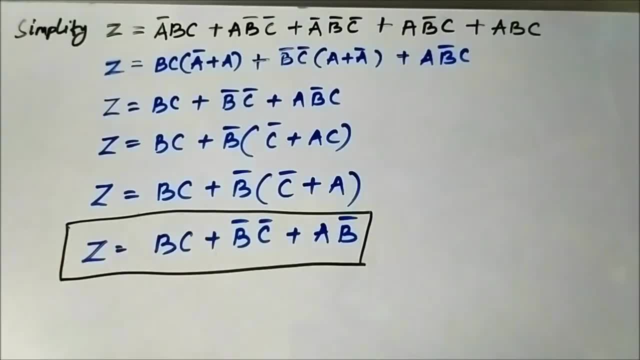 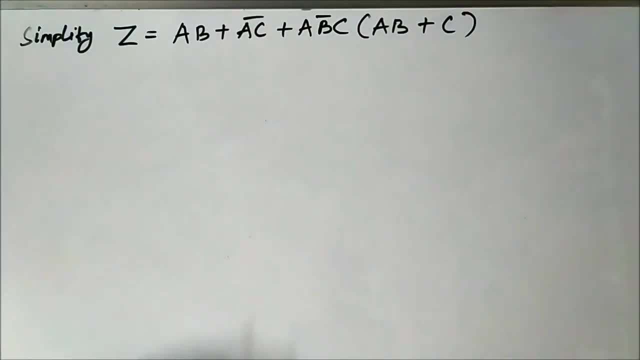 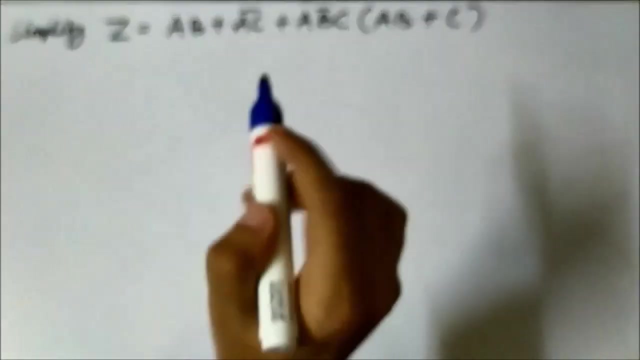 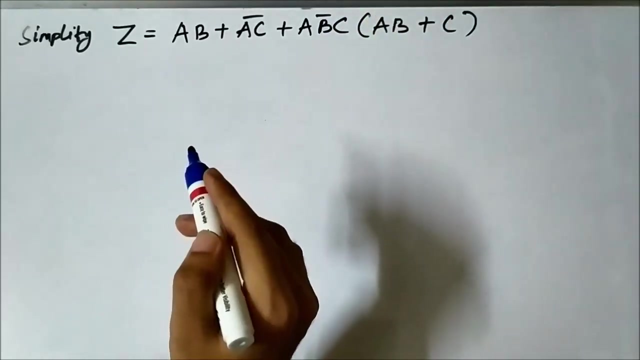 Okay, So here this is the simplified expression. So here we are with another Boolean expression which we have to simplify by applying the Boolean simplification rules. So the expression is this: Okay, So, So now let us just open up this bracket. I think we can eliminate a lot of terms, because 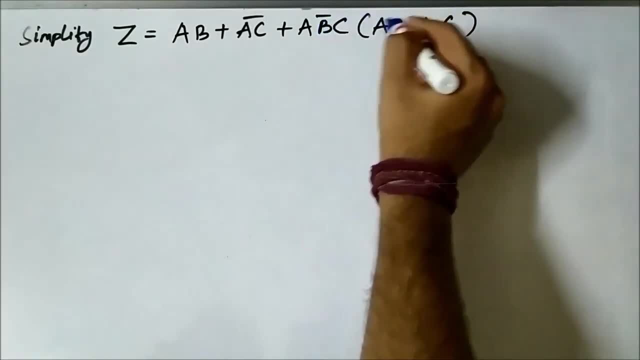 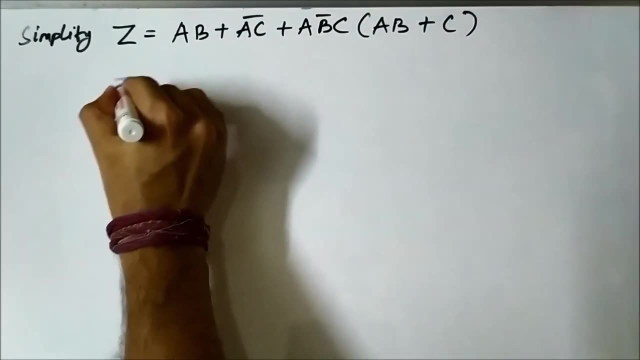 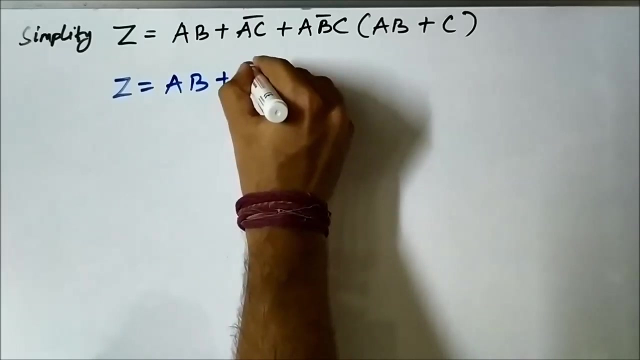 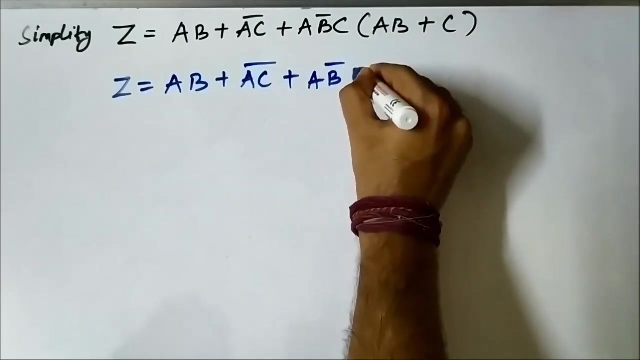 here b bar is present and here b is present. So when it will get multiplied we will get the 0 term. So let us open up this bracket first. So z is equal to a, b plus a c whole bar. opening up the bracket we will get a b bar, c, a b plus. 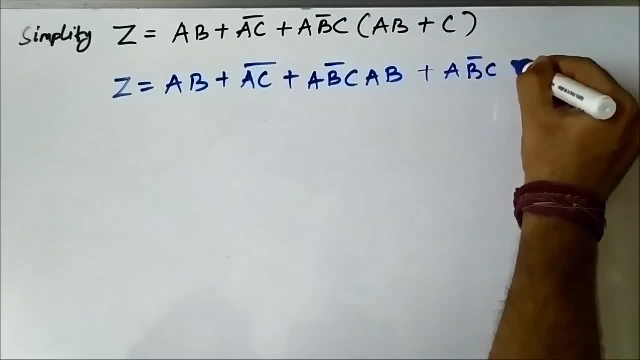 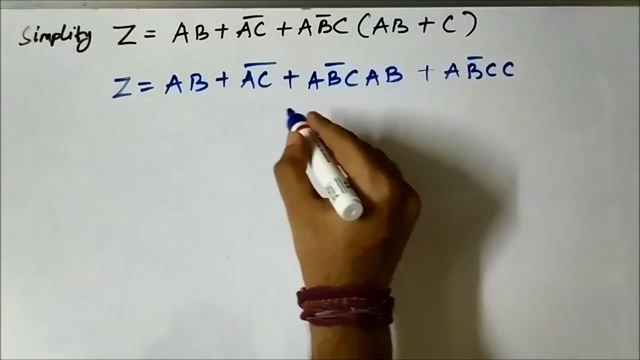 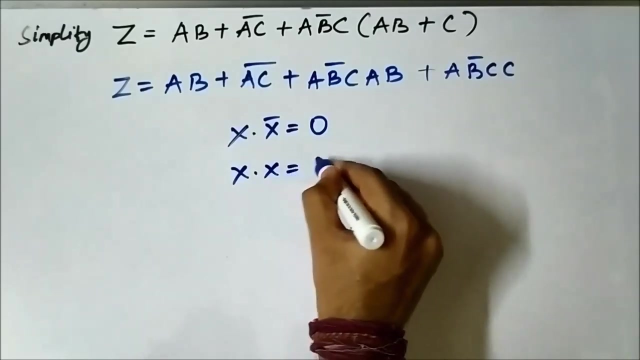 a, b, bar, c, c. So here the Boolean rules will come into play. this: So: any Boolean term anded with its complemented version will give us 0 and any Boolean term anded with the same Boolean term will give us the same. So two same Boolean, equal Boolean terms anded together will result in the same Boolean term. 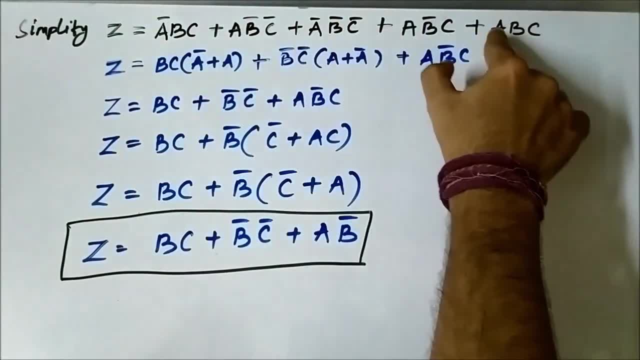 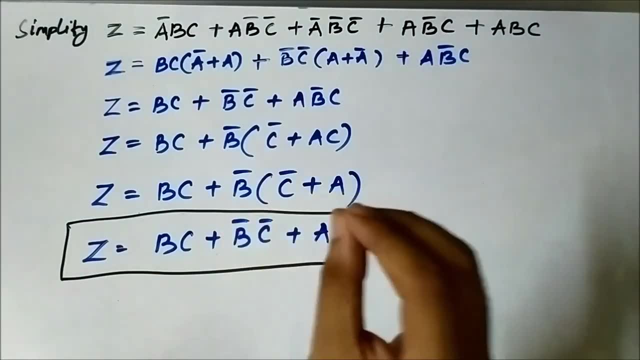 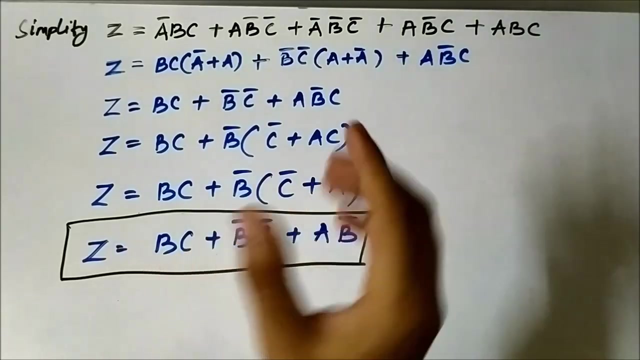 you have to take care is to identify common terms In the Boolean expression, then arrange them in a particular manner where you can apply the Boolean algebra rules, the simplification rules. So for that you have to be crystal clear about the rules, You have to remember them. Then keep on simplifying, keep on identifying. 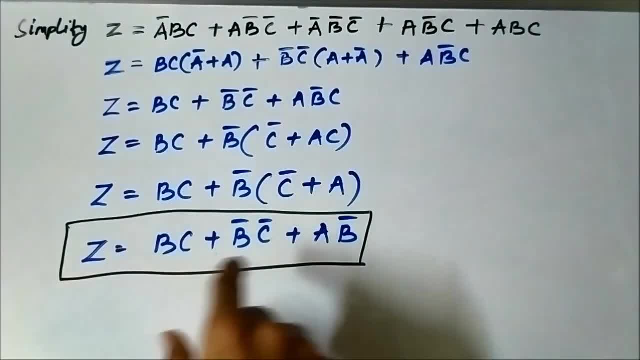 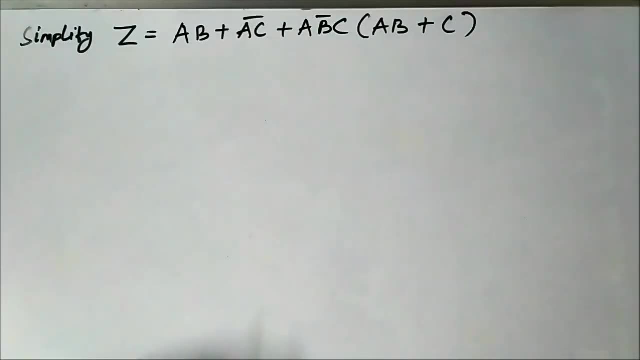 the patterns, keep on identifying the common terms until you get at a simplified reduced expression. So here, this is the simplified expression. So here we are with another Boolean expression, which we have to simplify by applying the Boolean simplification rules. So the expression. 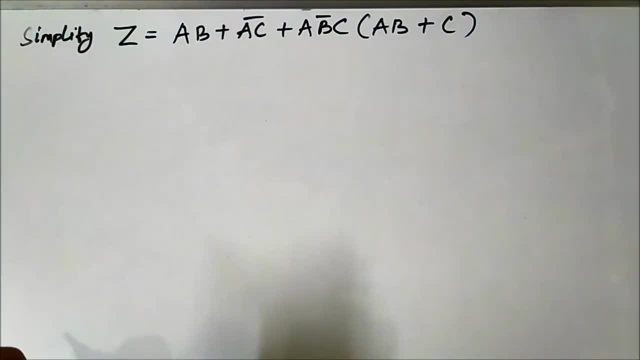 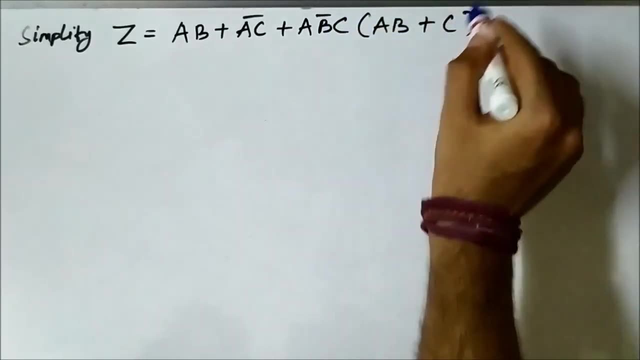 is this. So now let us just open up this bracket. I think we can, we can, we can write this Now: c bar, No, that means a whole Okay, because there are a lot of to consider. So whether, if we look at this circle there, 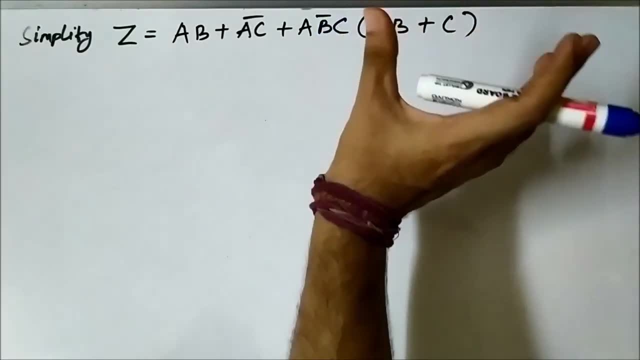 should be One spsan number, whether if we write a full number it should create the whole term. So here we can eliminate a lot of terms, because here b bar is present and here b is present, So when it will get multiplied we will get the zero term. So let us open. 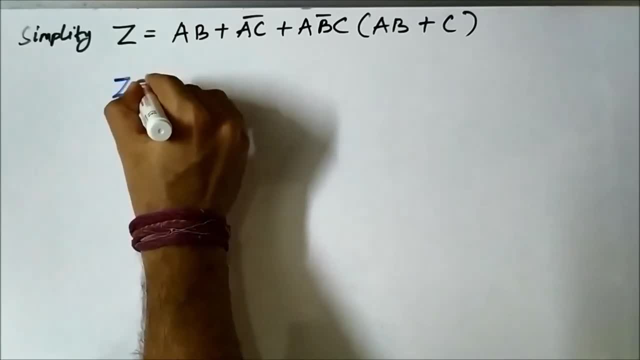 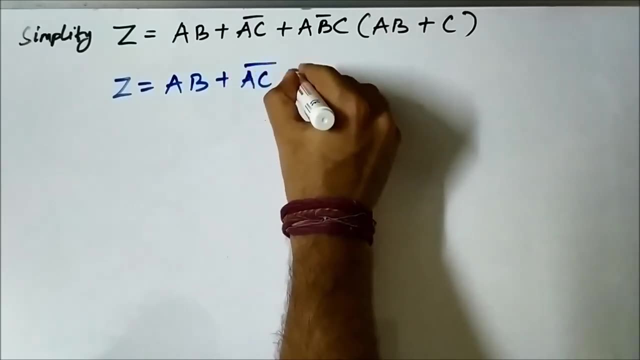 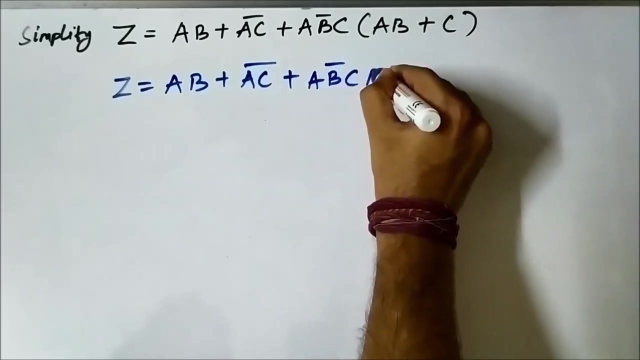 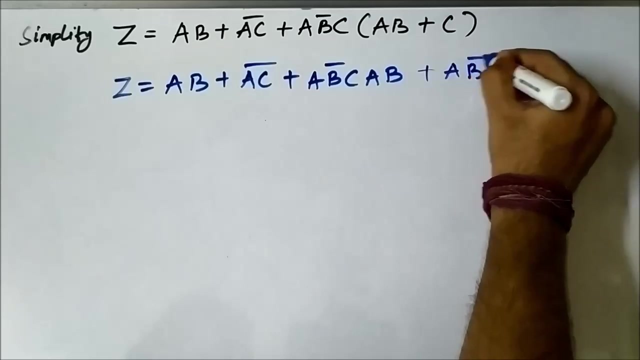 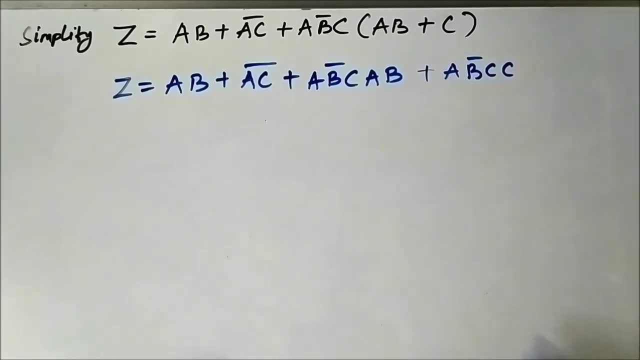 up this bracket first. So z is equal to a, b plus a c, whole bar. opening up the bracket will get a b, bar c, a b. So example and case 1.. plus a, b, bar c, c. okay, so here the boolean rules will come into play. this: 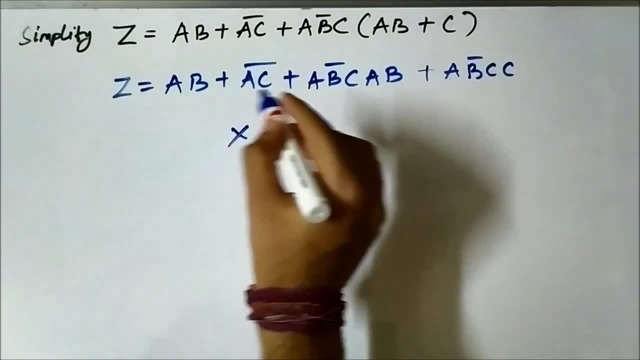 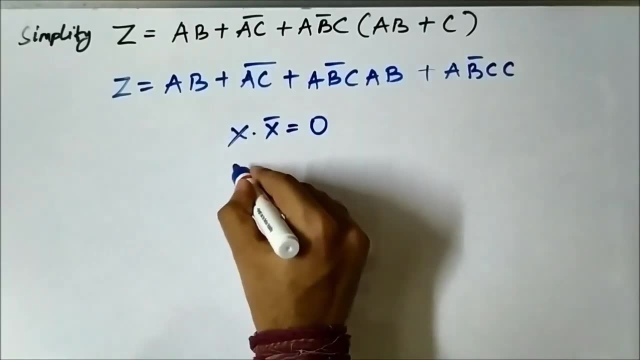 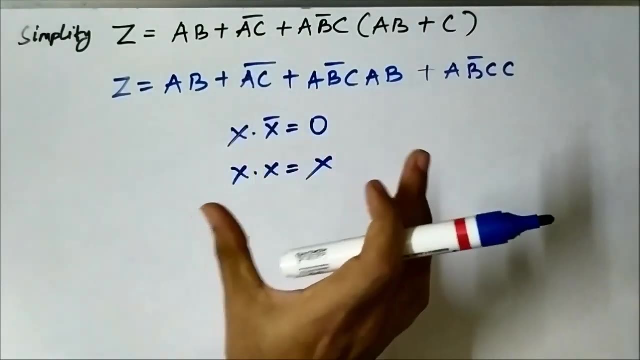 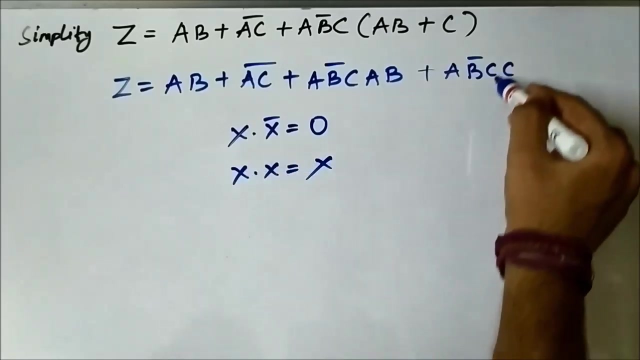 any boolean term anded with its complemented version will give us zero, and any boolean term anded with the same boolean term will give us the same. okay, so two same boolean, equal boolean terms anded together will result in the same boolean term, so this rule will be applicable. 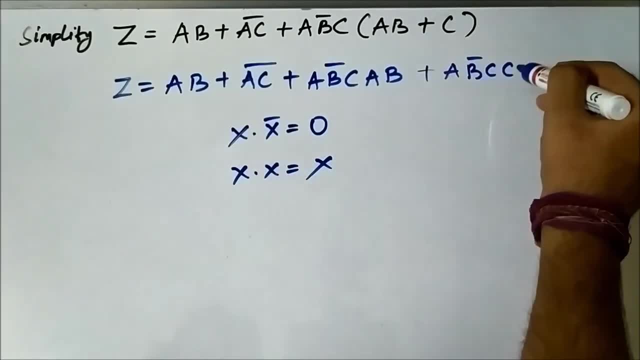 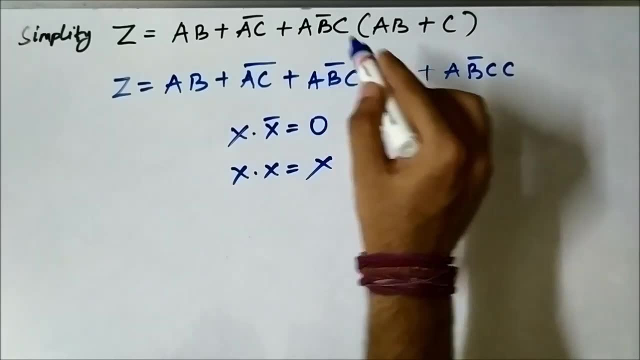 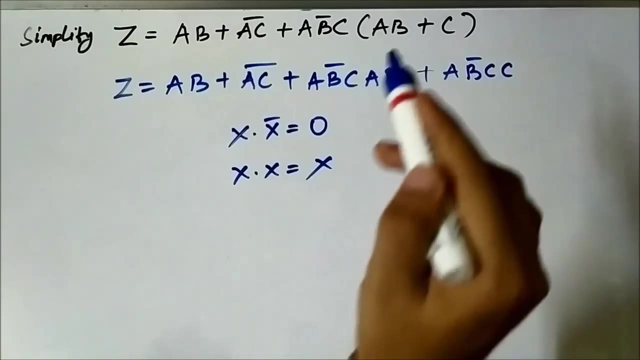 So this rule will be applicable here: c into c will become c, and this rule is applicable here Here: b bar into b is 0. Again, I repeat here: when I say multiplication, or into, it means and operation, and when I say plus, it means or operation. 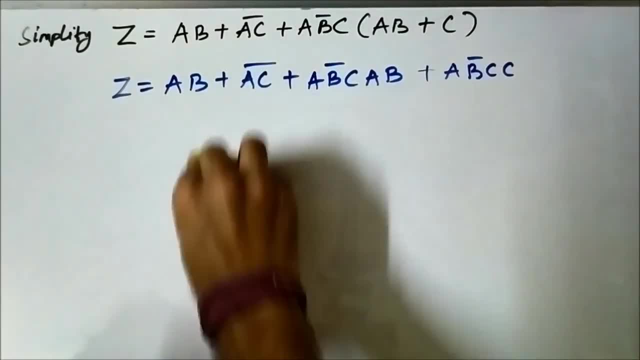 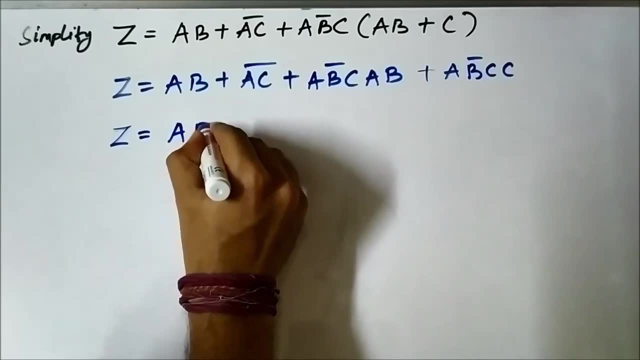 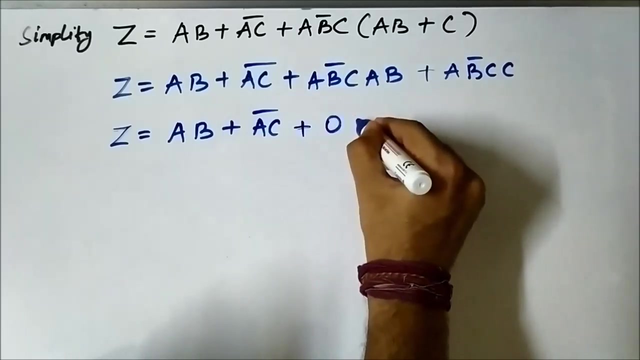 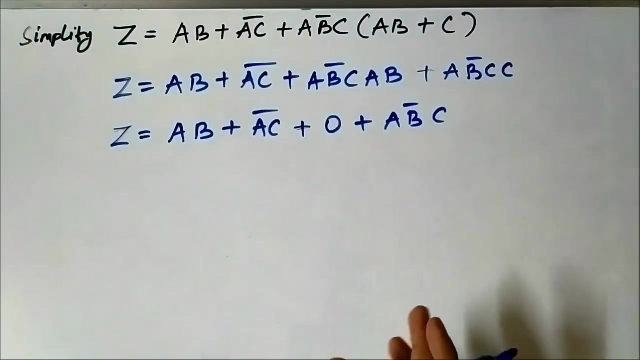 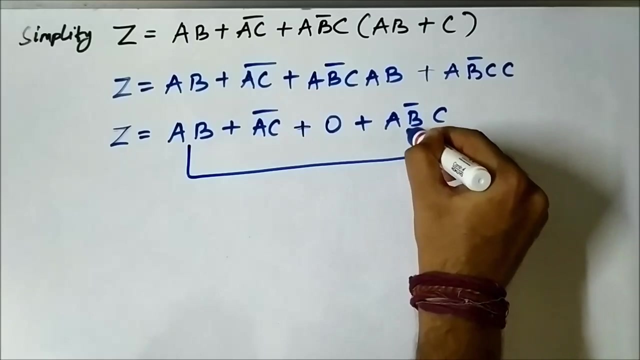 So let us apply these two rules here. So here it will be: z is equal to a b plus a c, whole bar. Here this whole term will become 0 plus a b bar c, a b bar c. Now. so see, here in this term and this term a is common, a is present, here a is also present. 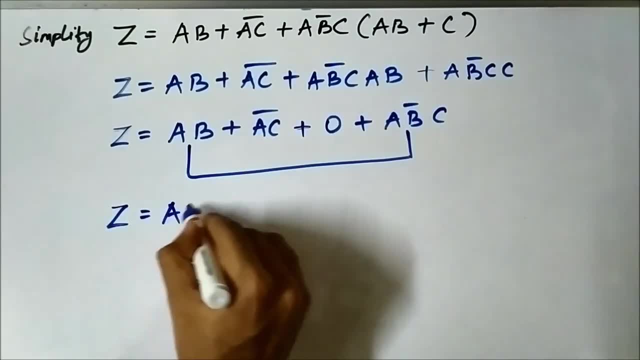 here. So let us take a common here, So it will become a into b plus b bar c. So this is common. So let us take common here, So it will become a into b plus b bar c. Now x is also common, so every information here also will be common. 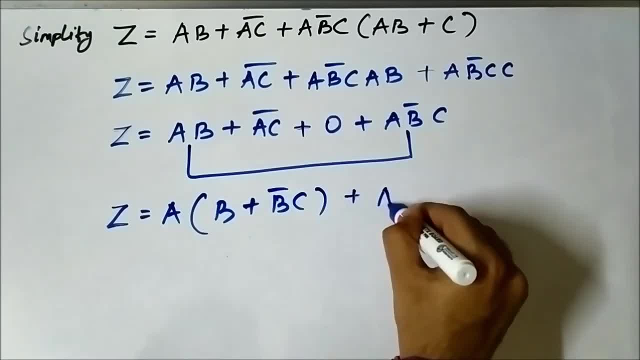 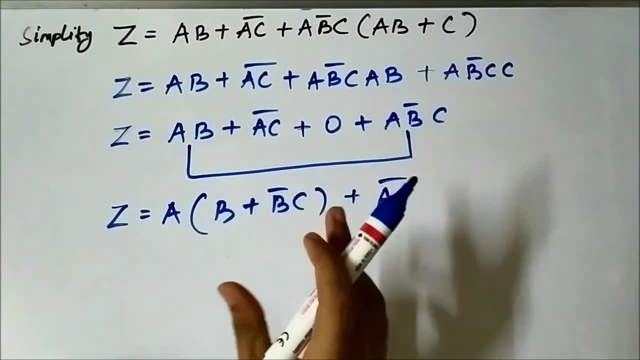 A- c whole problem here points to a through a plus b. Now again here another Boolean algebra rule will come into play, the absorption rule, which says: x plus x bar y is equal to x plus y. So we will apply this here. when we will apply this rule? 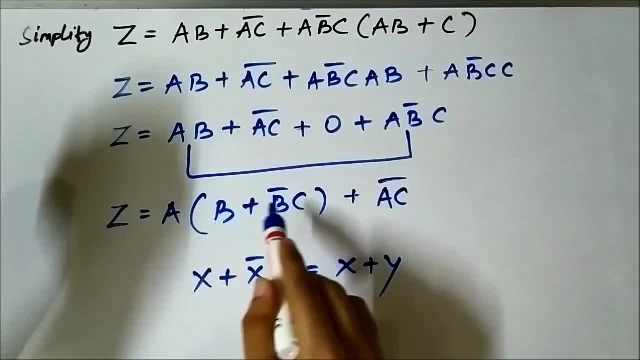 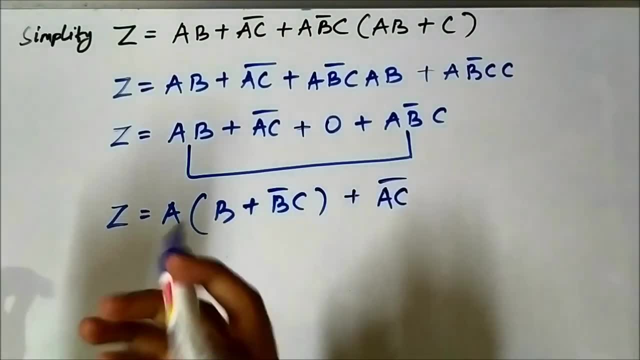 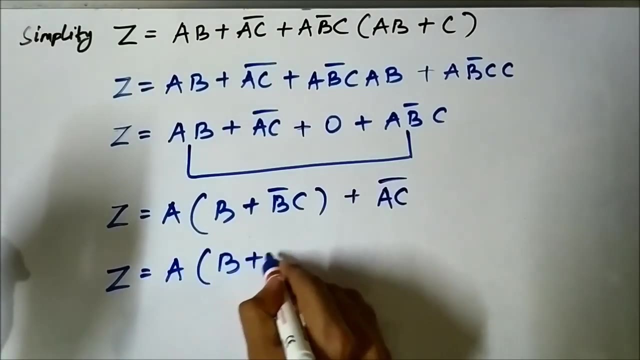 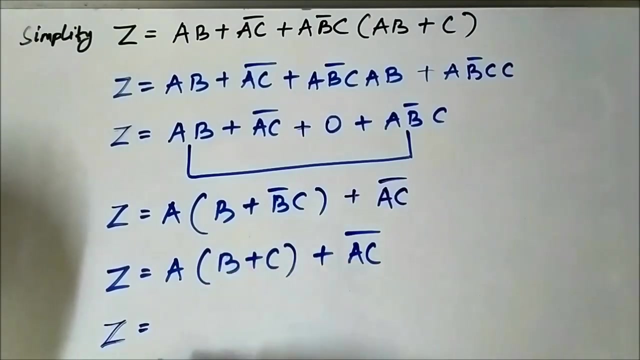 It will become c into x. Let us take a local Y, b plus c, b plus b, bar c will become b plus c. okay, so let us apply it here. so it will become z is equal to a into b plus c plus ac whole bar. okay, let us open up the bracket. it will become: 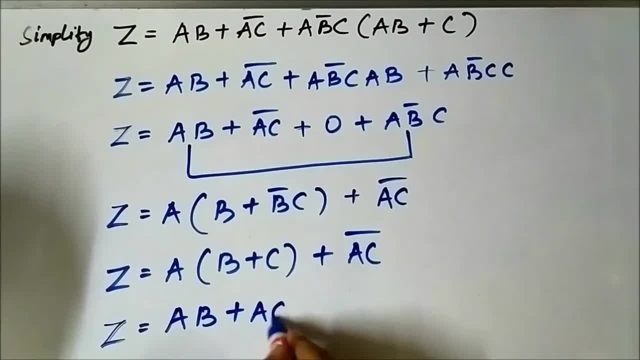 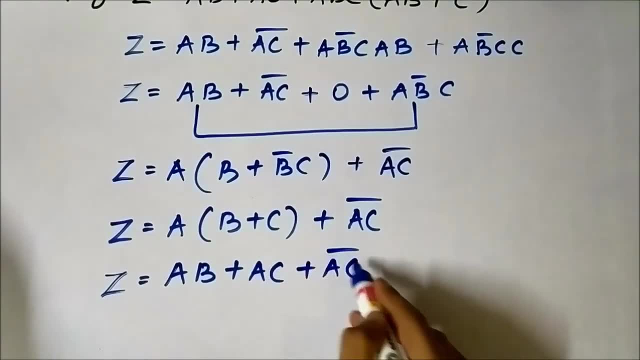 a b plus a c plus a c, whole bar. okay, these two terms, a c plus a c, whole bar, we can just apply this rule here: x plus x bar is equal to one. any boolean variable, orred with its complemented version, will give us one. okay, so here a c plus a c. 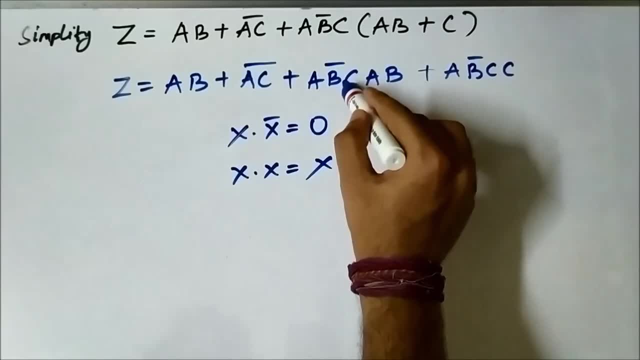 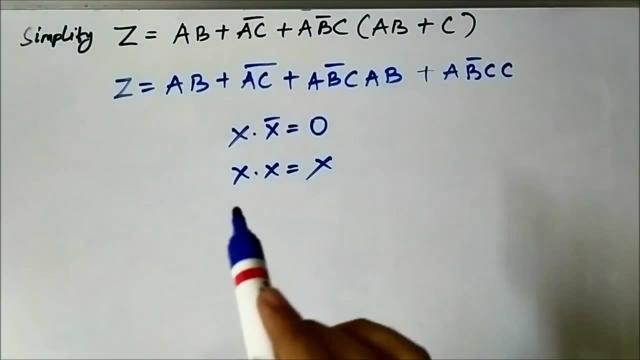 here c into c will become c, and this rule is applicable here. b bar into b is zero. again, i repeat here: when i say multiplication, or into, it means and operation, and when i say plus, it means or operation. okay, so let us apply these two rules here. so here it will be: z is equal to. 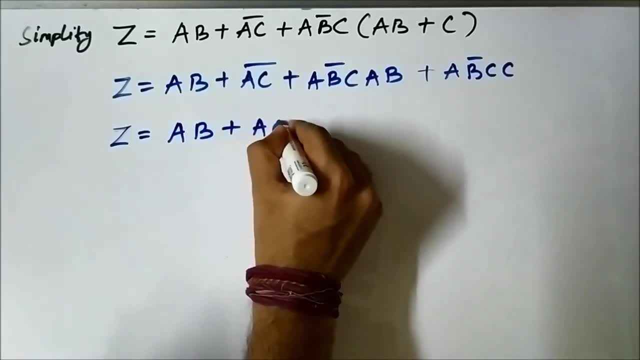 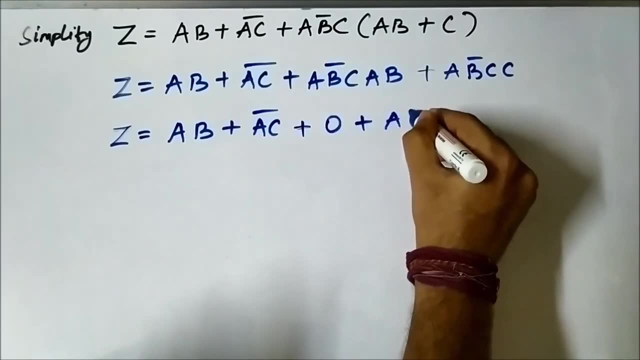 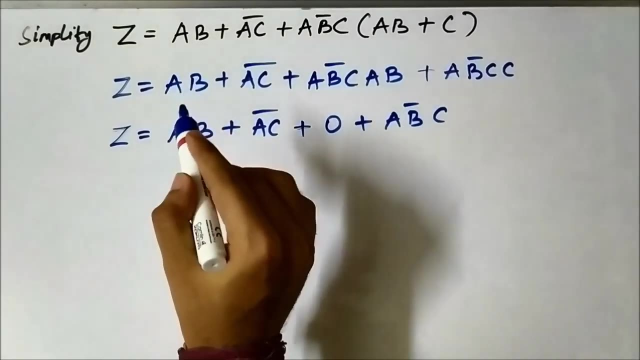 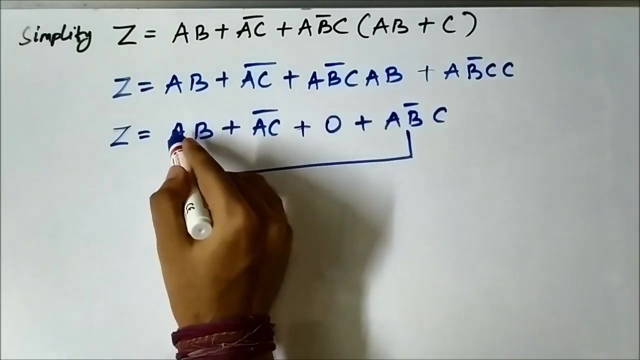 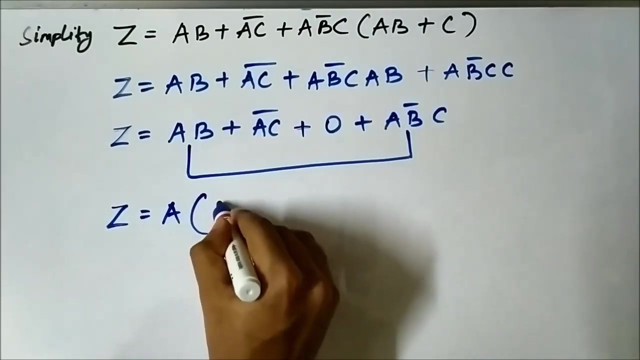 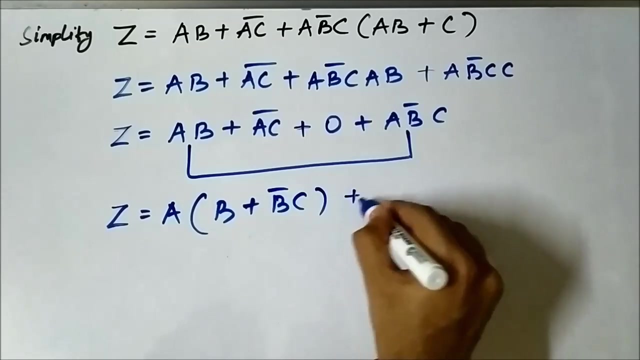 a b plus a c whole bar here. this whole term will become zero plus a b bar c. okay, a b bar c now. so see here in this term and this term, okay, a is common, a is present here, a is also present here. okay, so let us take a common here. so it will become a into b plus b bar c plus a bar a c whole. 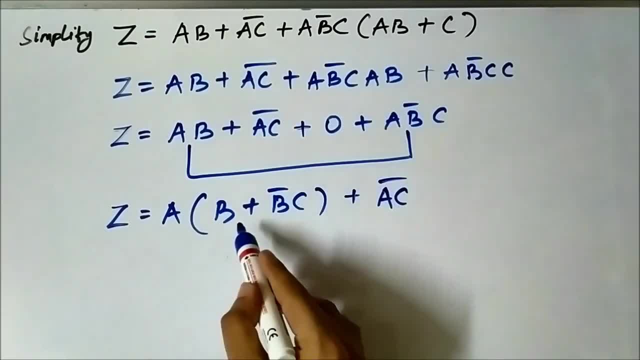 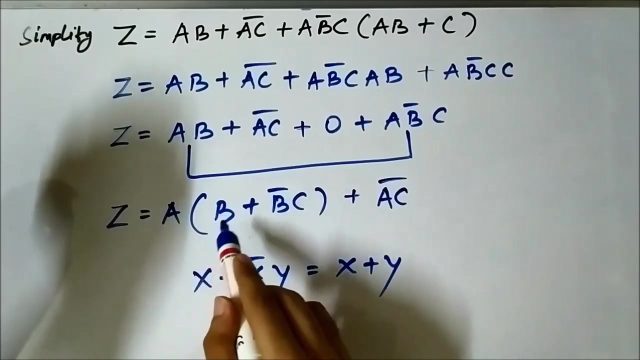 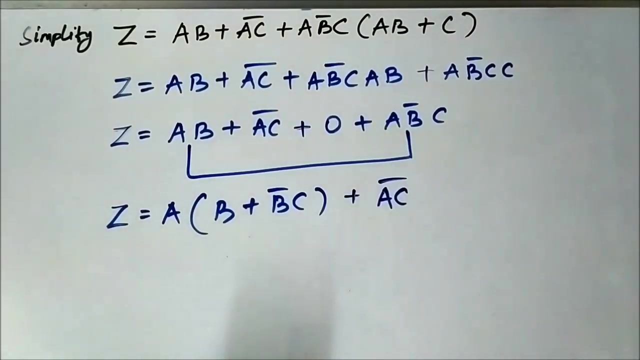 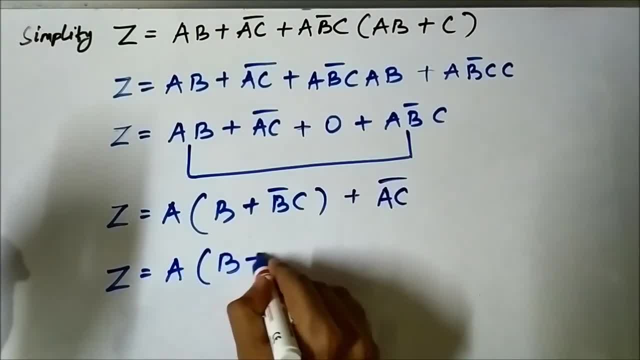 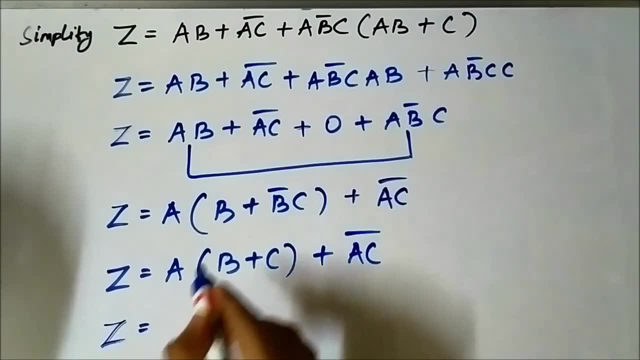 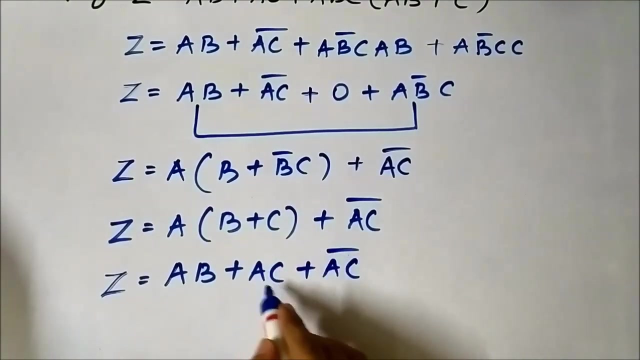 to a into b plus c plus a c whole bar. okay, let us open up the bracket. it will become a, b plus a c plus a c whole bar. okay, this two terms, a c plus a c whole bar. we can just apply this rule here: x plus x bar.